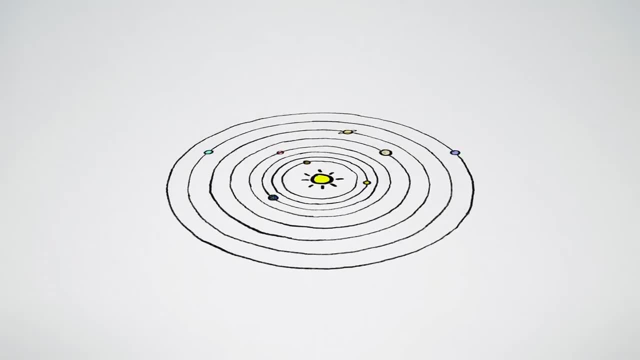 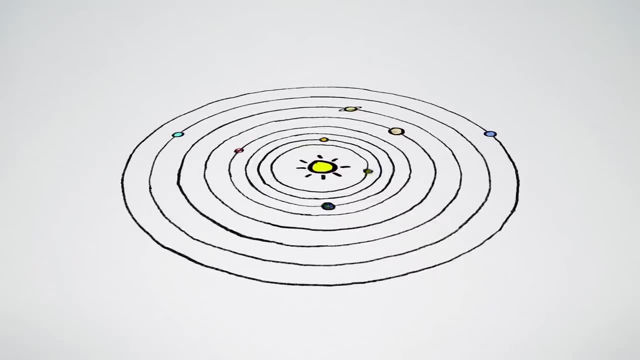 both a totally not-scale caricature and yet also represents the very real idea that the planets all orbit the sun in roughly the same plane and that some are farther out and some are closer in. and if it's animated, we get to see that the closer planets complete their 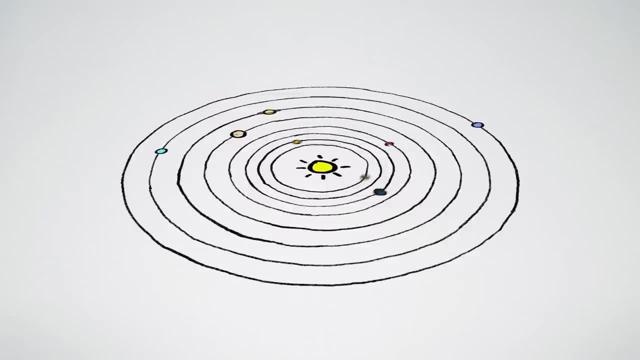 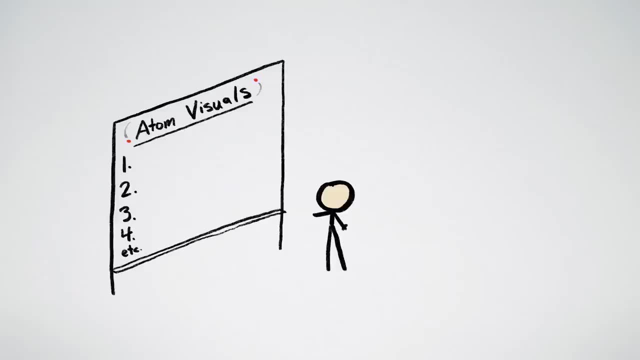 orbits more often. It's a nice picture and that's what I want for atoms: A good picture. There are a few things I'd like that picture to get across. some of them because they're important for the physics of atoms, and some of them because they're questions my brain. 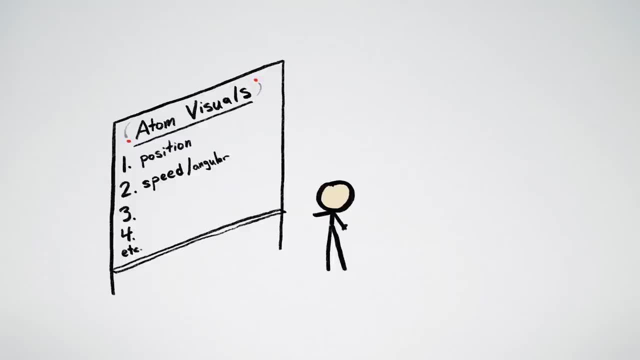 wants answers to Like: where is the electron? How fast is it going? How much energy does it have? How big is this picture relative to other pictures? Of course, the wave-particle nature of quantum mechanics means some of these ideas like: 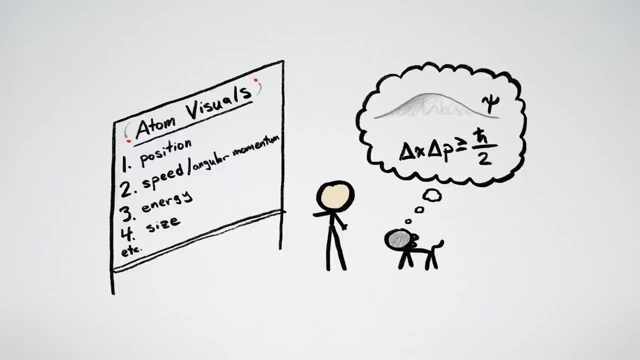 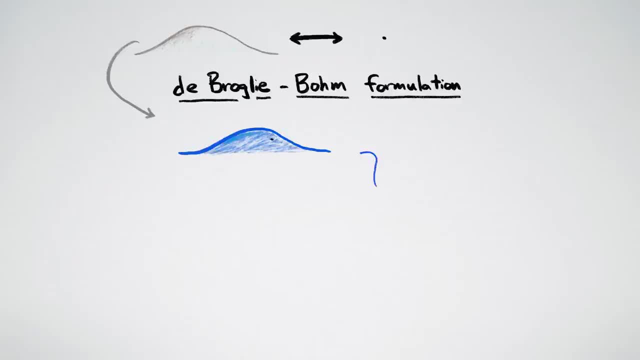 the electron's position don't translate exactly from our everyday intuition to the atomic scale. But there is a way of thinking about wave-particle duality where you can picture the wave-function as a bunch of water and the particle as a speck of dust. in that 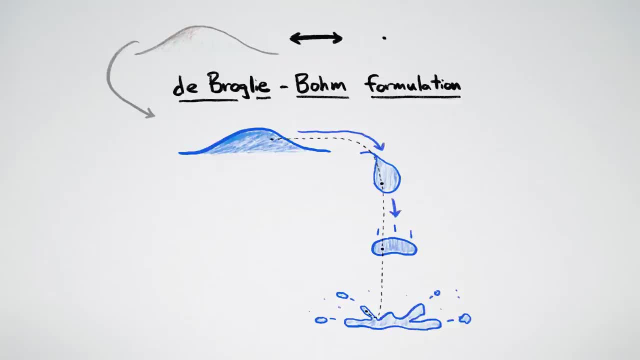 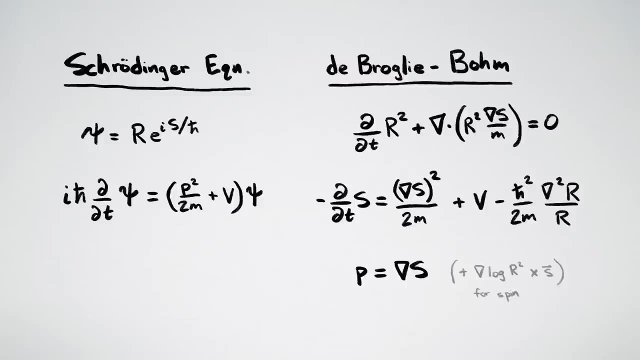 water. The particle is mostly guided by where the water goes and the water is guided by the equations that determine how water behaves depending on its circumstances. And if you apply the mathematics of that idea to atomic orbitals and then render it in three dimensions, 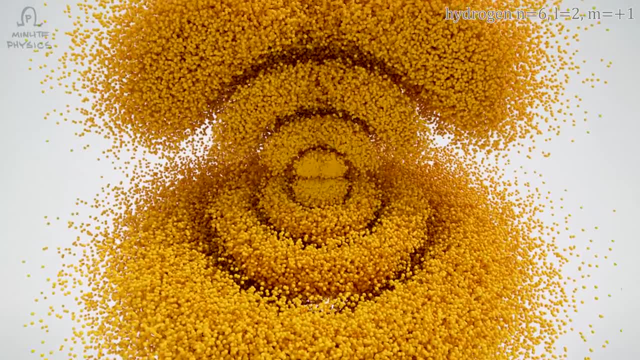 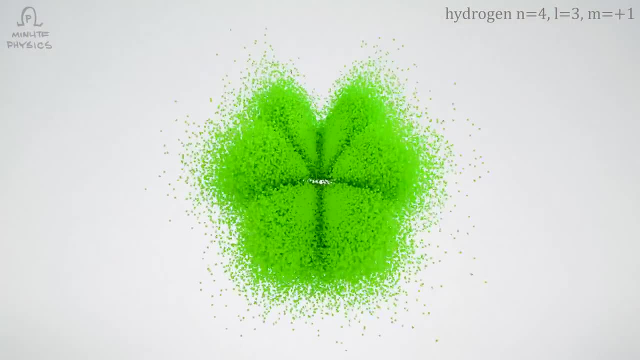 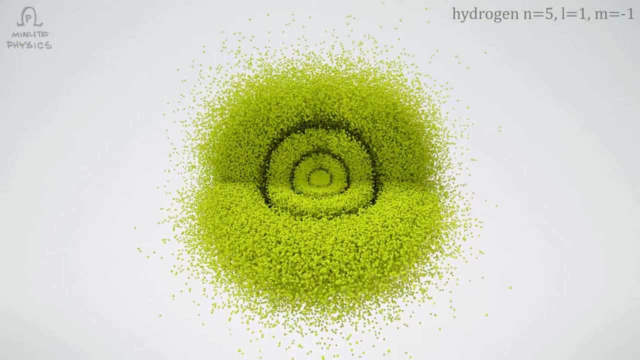 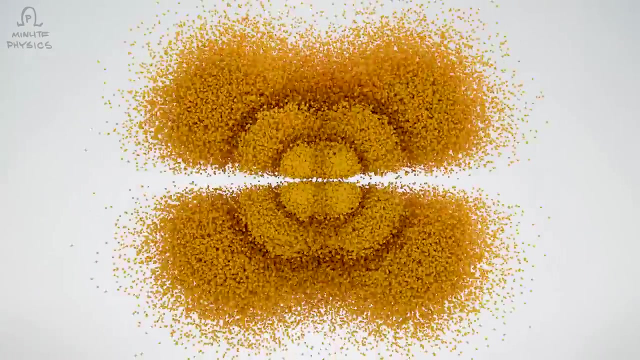 here's what you get. Isn't it beautiful? Here's another, And another, And another, And another. In fact I made a bunch of these And they're all mesmerizing and beautiful. and isn't the ground state of the hydrogen atom? grist, so cute. And aren't the excited states so? 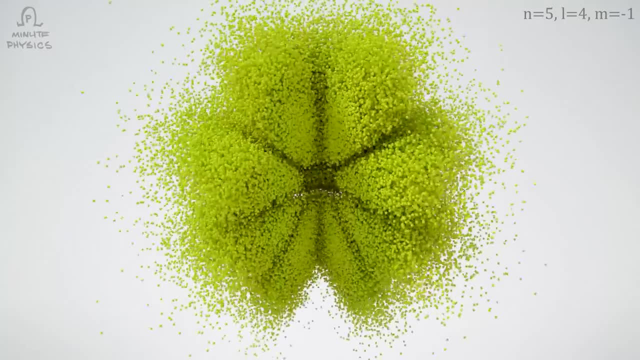 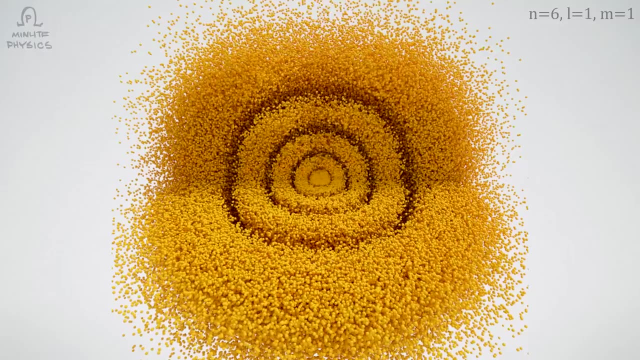 majestic. There's so much structure and detail in them. I just love it. You can see patterns in the orbitals and you can get a sense that they actually are orbitals. I mean, something is orbiting. There's boundaries that empty the jelly man. 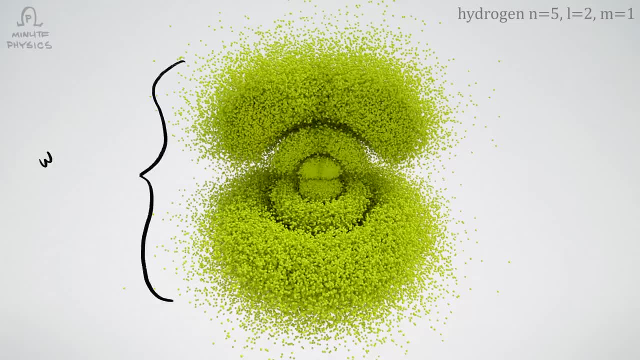 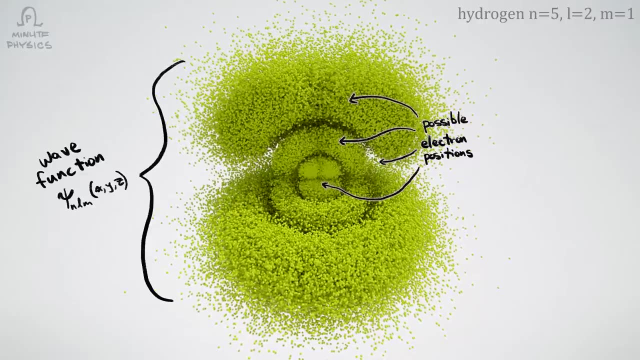 Okay, so I do have to be clear. the dots don't each represent a separate electron. The whole collection represents the wave-function of a single electron, and individual dots represent all the places that electron could be. A higher density of dots means a higher probability. 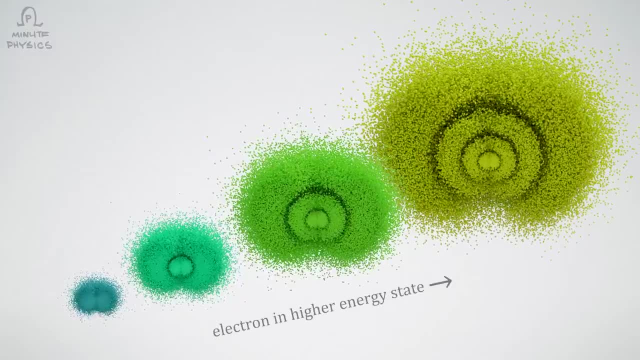 of the electron being there, the bigger orbitals are the ones with higher energies, because electrons with more energy are more likely to be far away from the nucleus. The motion of the dots is showing the這裡 with the lower horn of the far end of the자가, The. 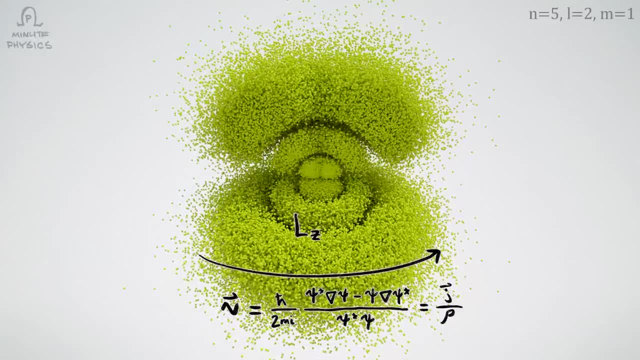 response of that wave-function. its energy mass is showing the flow of the wave-function and its density corresponds to an extent with its angular momentum. Though they're ever-so-ницыca-fine theave above those only aólng the energy mass, And whilst they're tame enough to publicly